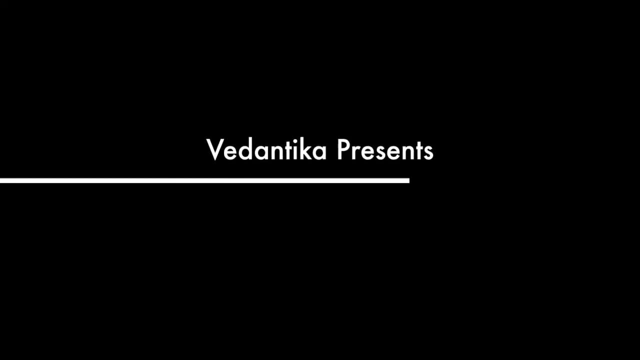 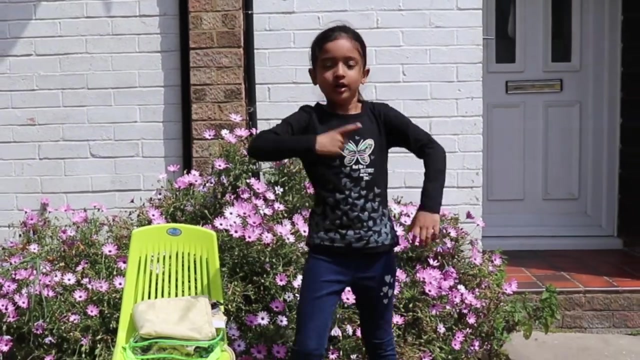 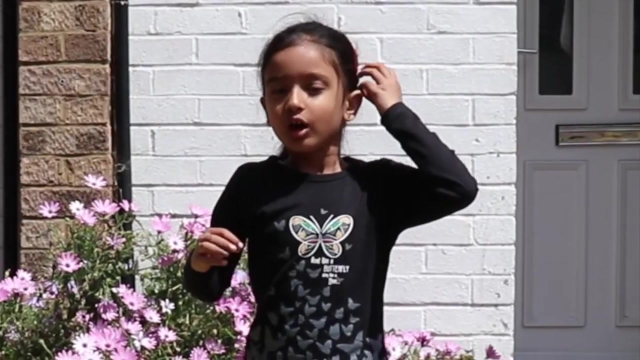 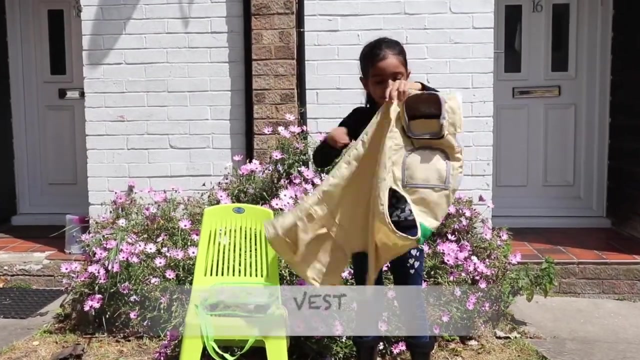 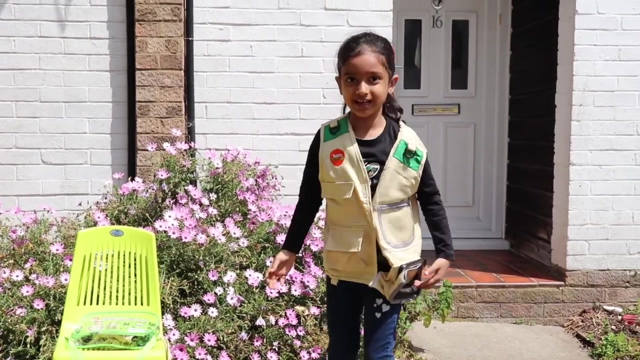 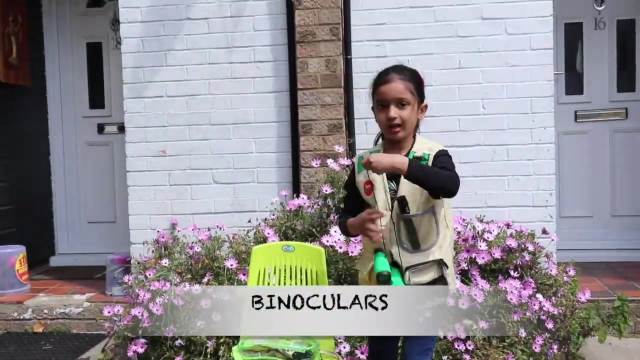 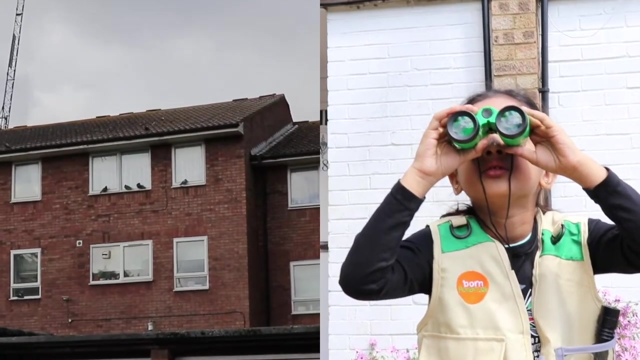 Hello, I'm Dora, not an explorer, yet I needed a clover kit to start my exploration. Hope you will join in on my journey to unlock some extra parts. My best Pocket for everything: Flashlight, Binoculars. 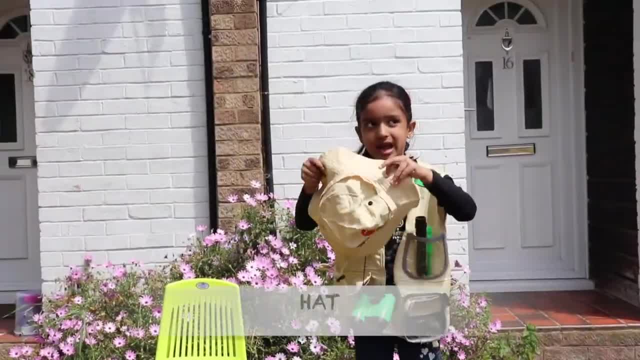 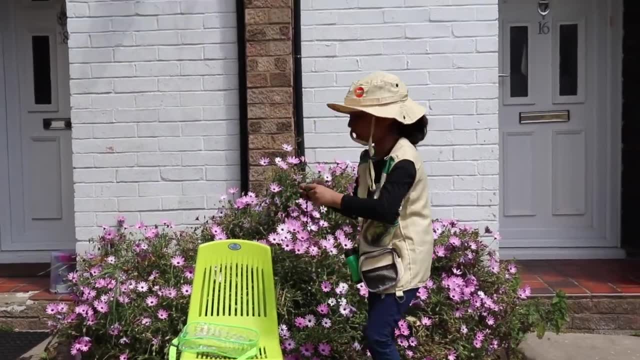 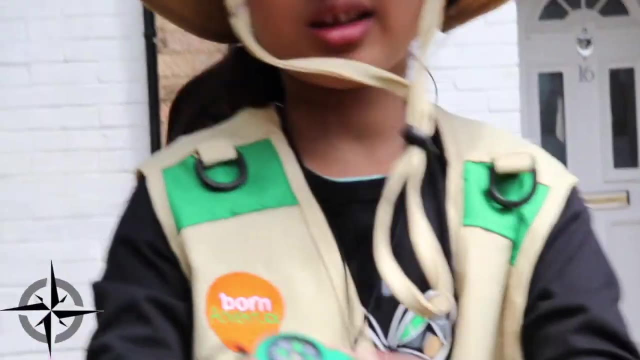 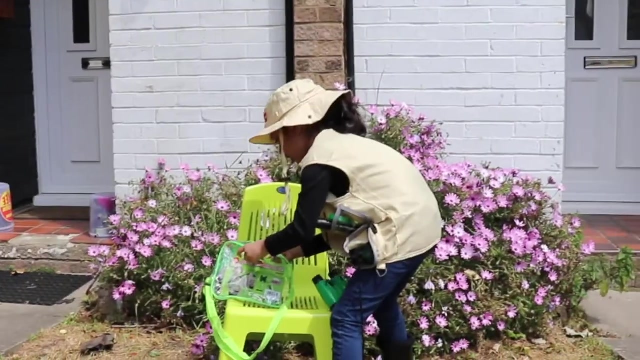 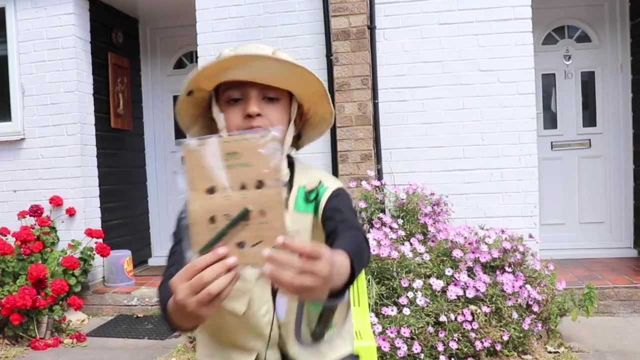 My manaflying blouse, My hat, Basketball, My whistle. It has a compass too. North, South, East, West. My costume is the best. This is my exploration sheet. I have to find all these. I found an ant. 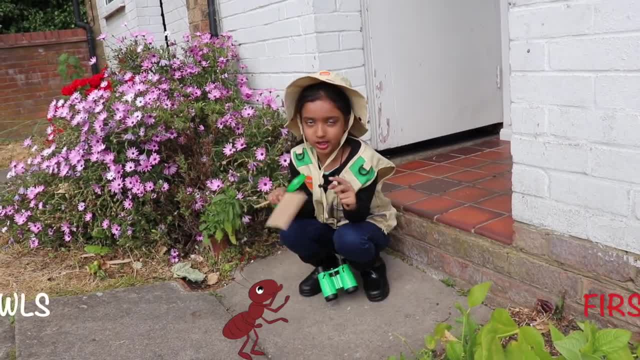 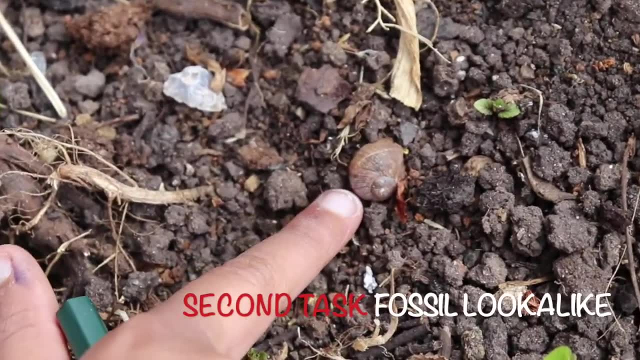 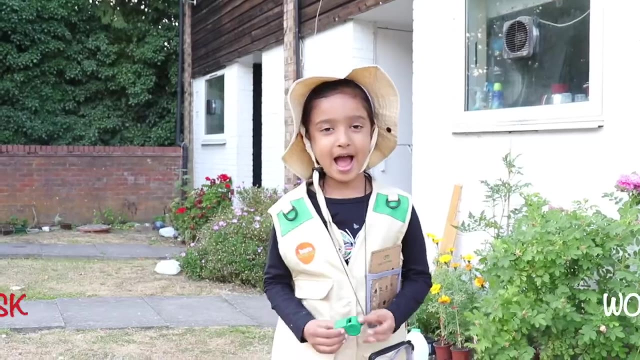 Do you know the ant was the longest living insect. I'm going to take it. I found a fossil. Did you know that snails live everywhere on the earth? I'm going to take that. I know where we can find some worms. 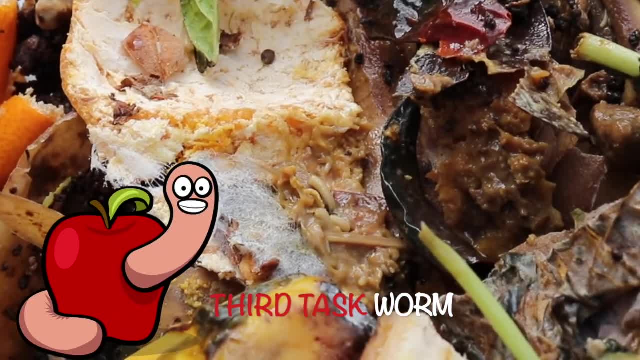 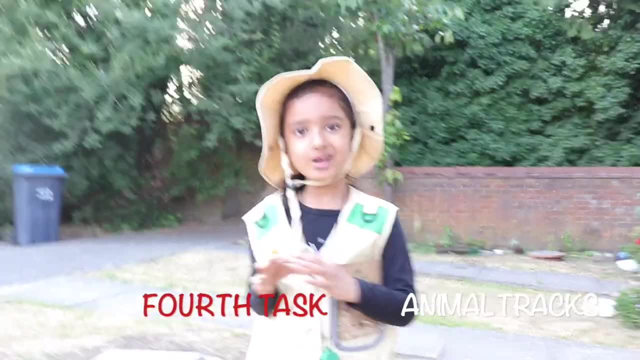 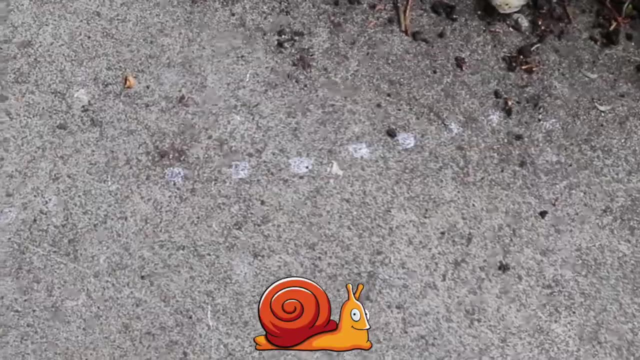 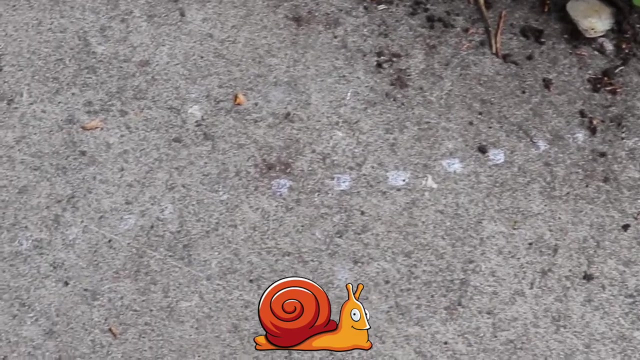 In the compost bin. They look yucky. Worms are good for the nature and the earth. Now I have to find the animal trail. I found the snail trail. I can't find the animal trail. I don't think there are any animal tracks around here. 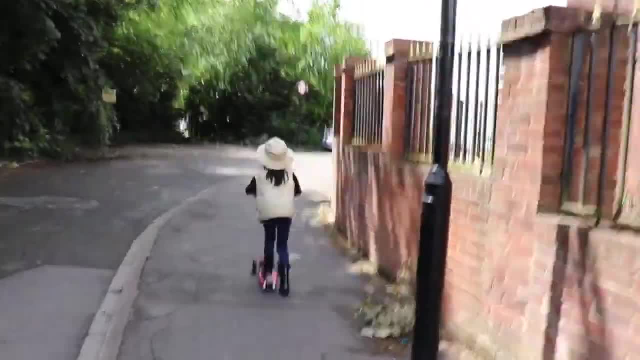 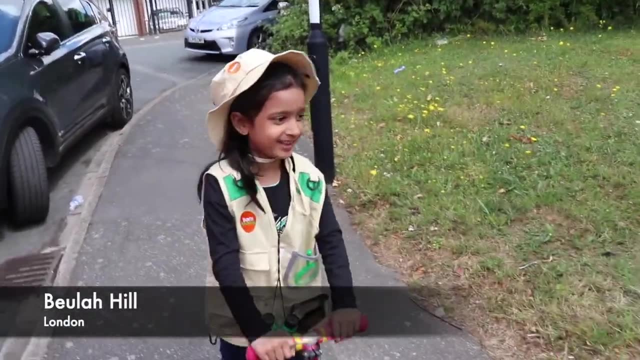 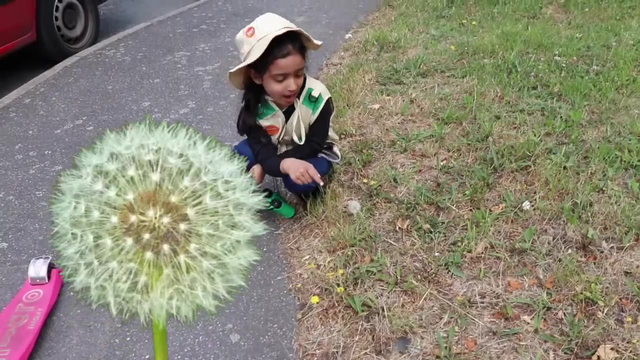 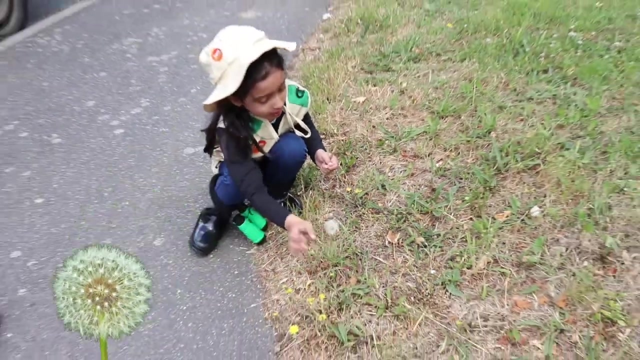 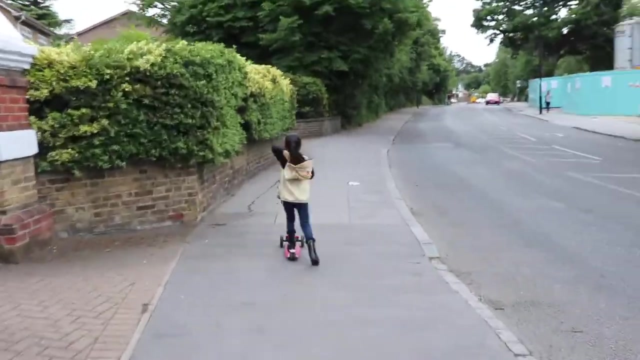 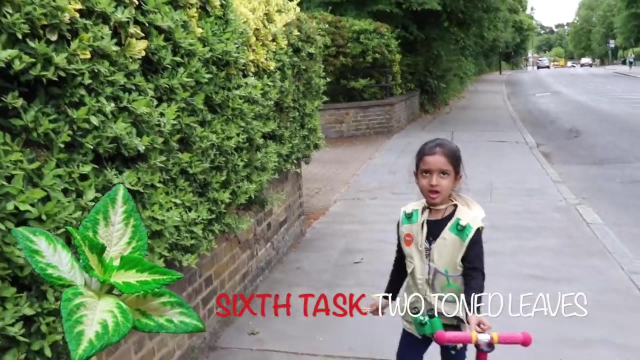 I found a dandelion. The snail present the stars and the other part present the moon. It looks like the stars. Look at the moon: It looks like a star, and moon Look a cute little leaf. We can't jump there because the tree is not going to let us. 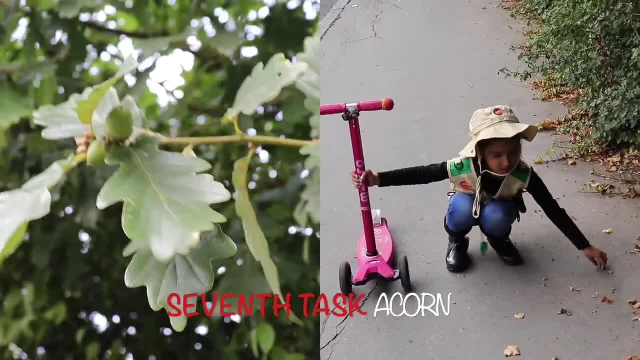 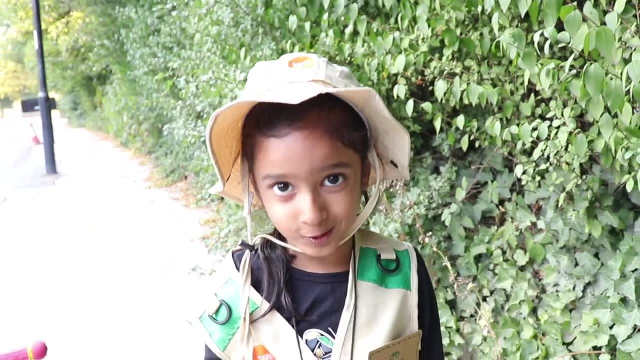 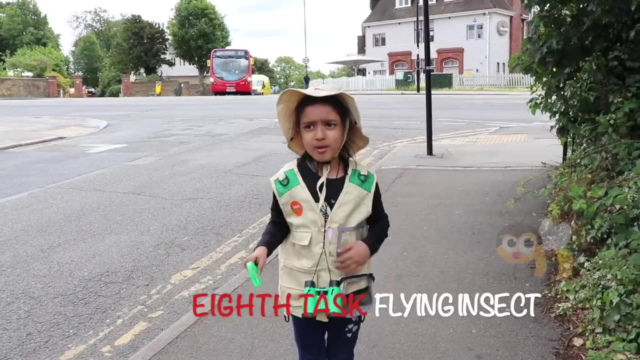 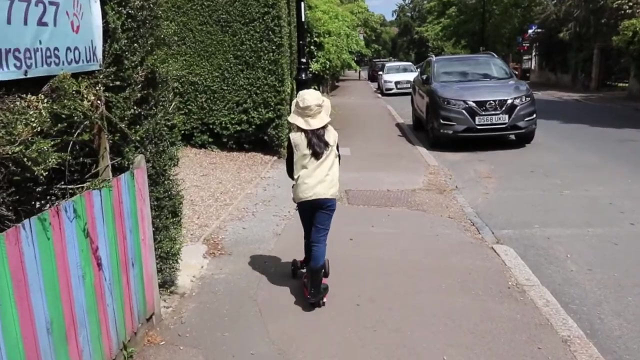 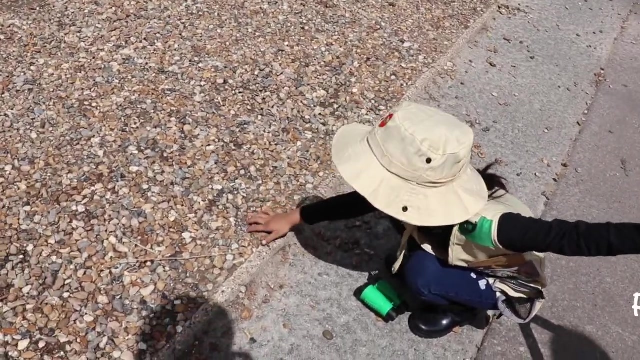 I found some acorns. Squirrel loves eating acorns. I found one bumble bee. Did you know that bumble bees hibernate underground? Look, I found so many pebbles. Door in my nest it says rock, But I. 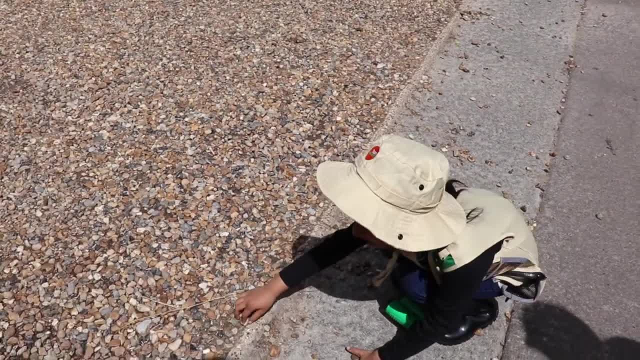 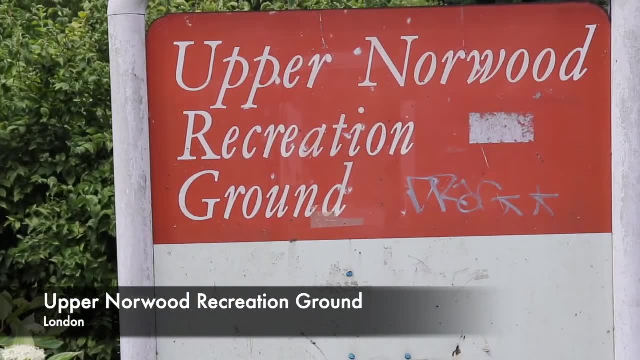 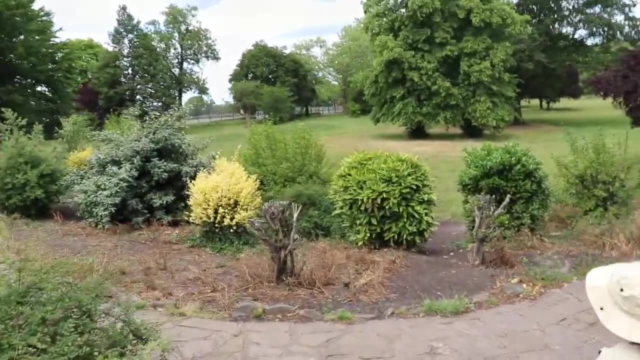 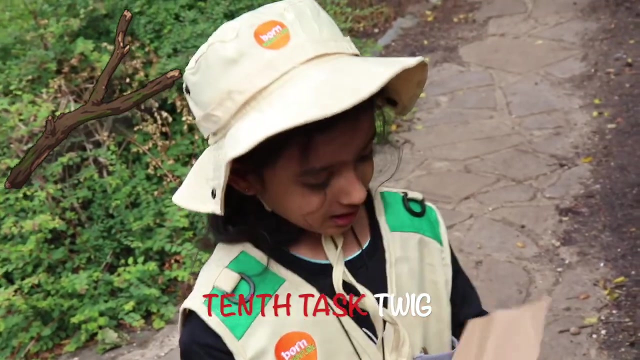 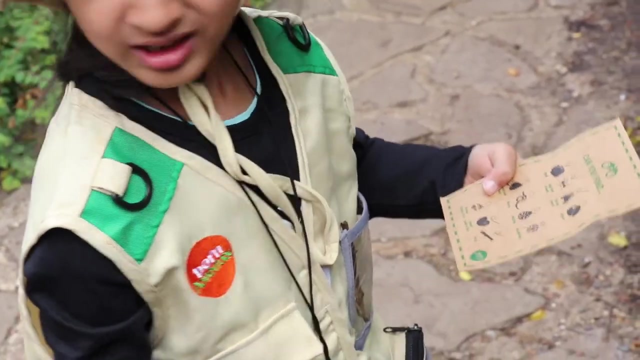 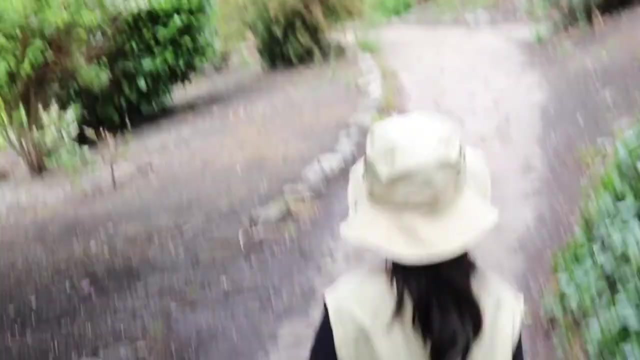 It says rock. It's okay, I can still take one pebble. Oh, I found a twig. I'm going to take it off in my challenge sheet. Challenge sheet. Oh, that's an acorn Challenge sheet. Challenge sheet. 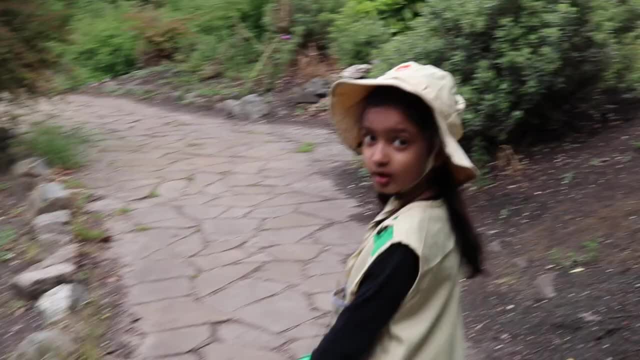 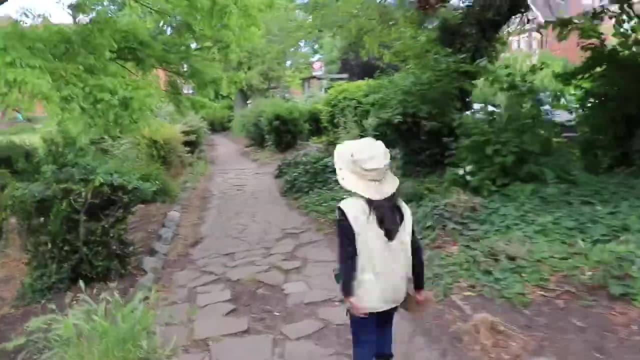 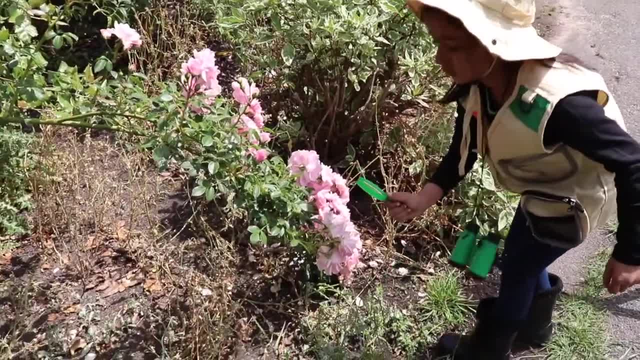 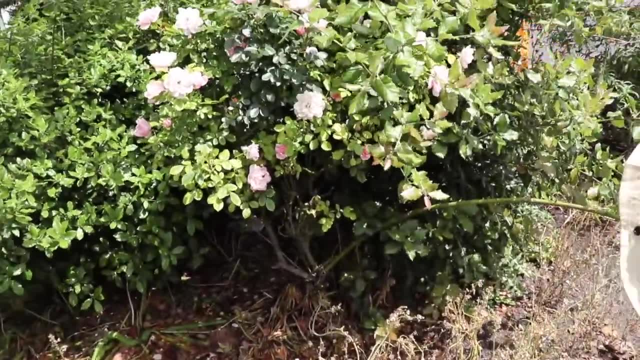 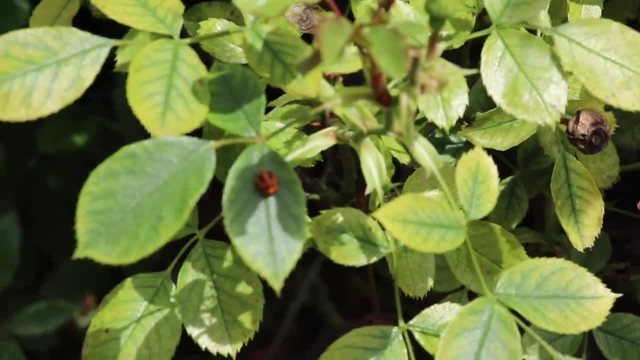 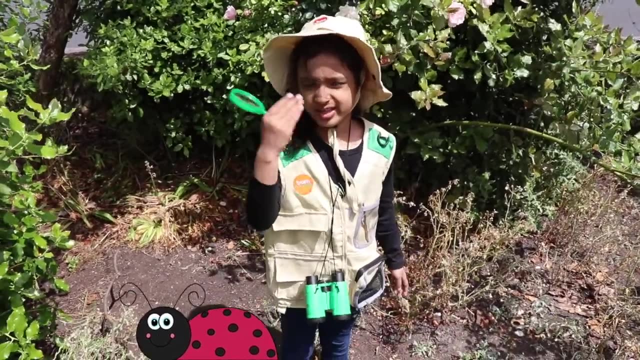